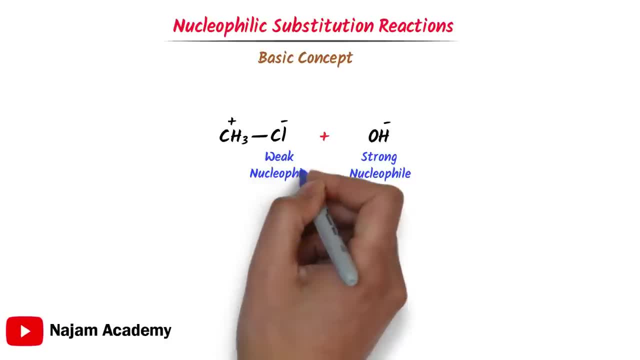 appears on this carbon. This chlorine is a weak nucleophile. Now listen carefully. This strong nucleophile will replace this weak nucleophile. Let me repeat it: This strong nucleophile will replace this weak nucleophile, Because we all know that strong nucleophile. 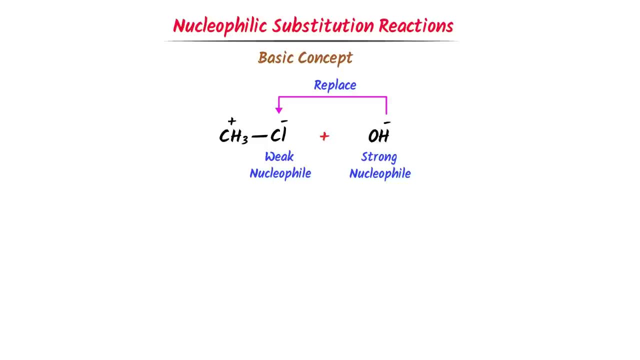 always rule over weak people. This is a substitution reaction, replacing one nucleophile by another nucleophile. That's why we call it nucleophilic substitution reaction. Therefore, we define the nucleophile substitution reaction as a type of organic reaction in which a strong nucleophile replaces weak nucleophile. is known as the nucleophilic substitution reaction. 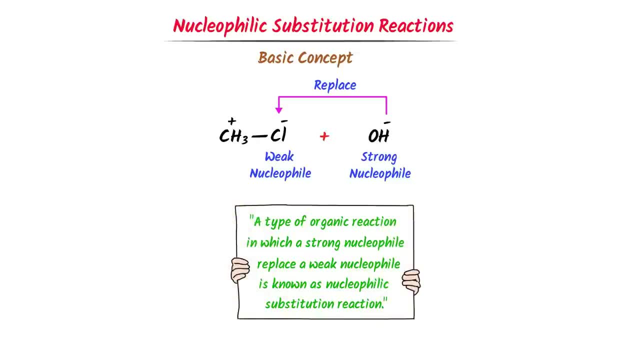 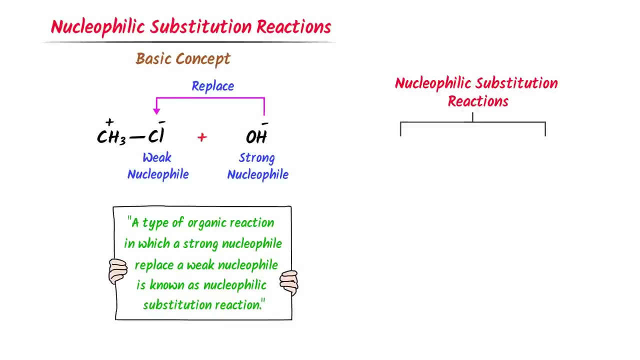 Let me repeat it: A type of organic reaction in which a strong nucleophile replaces a weak nucleophile is known as nucleophilic substitution reaction. Remember that there are two types of nucleophilic substitution reaction. The first is unimolecular nucleophilic substitution reaction, and we call it SN1 reaction, while 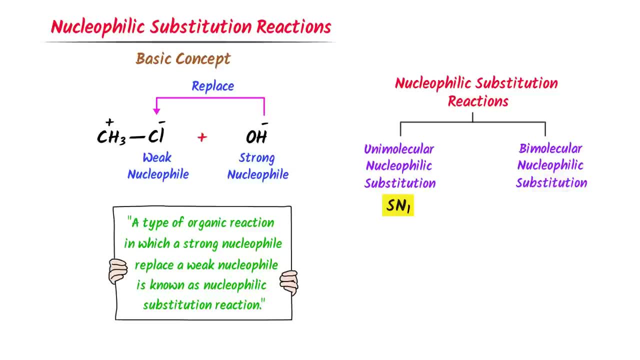 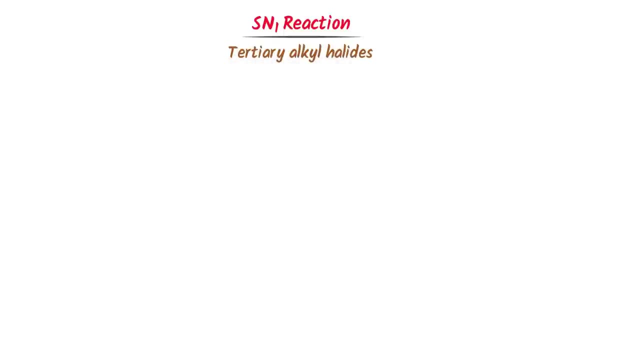 the second one is bimolecular nucleophilic substitution reaction, and we call it SN2 reaction. Thus noted down all these important points, Now let me teach you SN1 reaction. We know that tertiary alkyl halides favor SN1 reaction, So I take this tertiary alkyl halide. 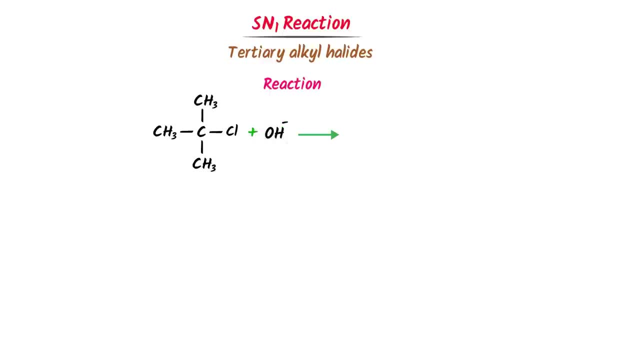 Now I place a nucleophile here. We already learned that this strong nucleophile will replace this weak nucleophile. As a result, we get this compound. Now what about the mechanism of SN1 reaction? Well, SN1 reaction occurs in two steps. 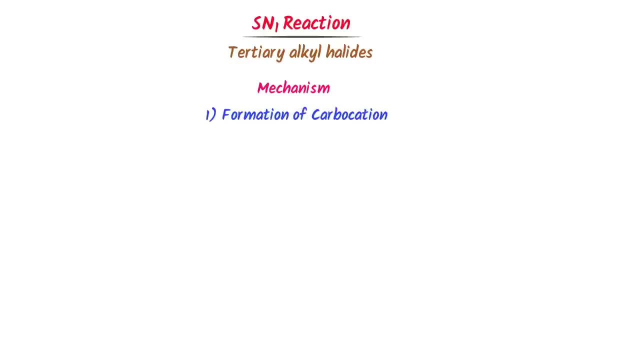 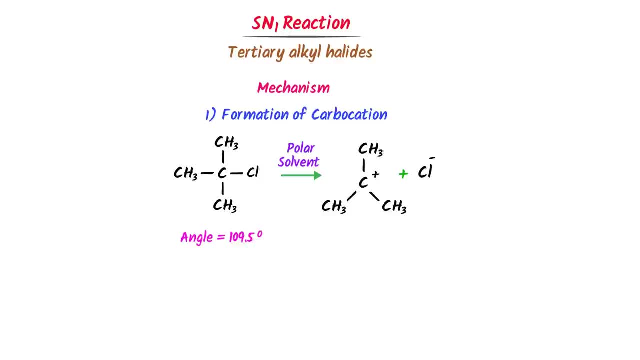 And this becomes a nucleophile, And this becomes a nucleophile. Here the angle between carbon atom is 109.5 degree, While there the angle between carbon atoms is 120 degree. Remember that first step is a slow step. Hence carbocation is formed in the first step. 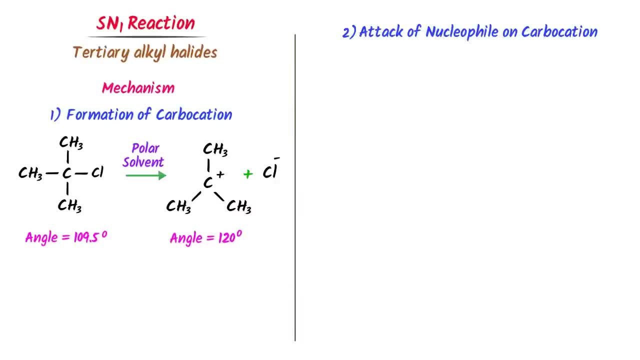 The second step is attack of a nucleophile on alpha carbon of carbocation. Now there are two possibilities of attack of a nucleophile. I take this carbocation and place it here. Let, in the first case, the nucleophile OH attack from the right side. 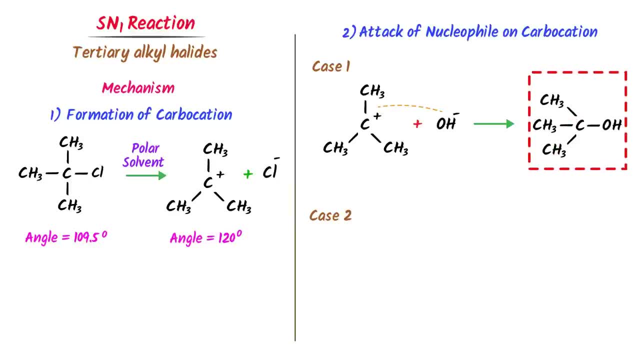 I get this compound Here. carbocation has retained its original shape- 50%- So we call it 50% retention of configuration. It means that this molecule has retained 50% of its original arrangement. In the second case, I take this carbocation and I place it here. Let this time. 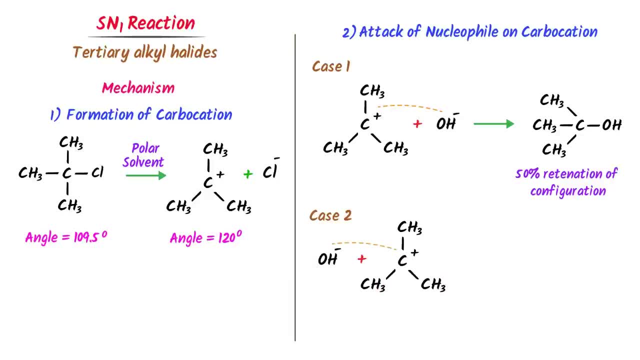 the nucleophile OH attack from the left side. As a result, we get this compound. We call it 50% inversion of configuration. Remember that SN1 reaction is faster in 3rd degree carbon, then 2nd degree carbon and then 1 degree carbon. 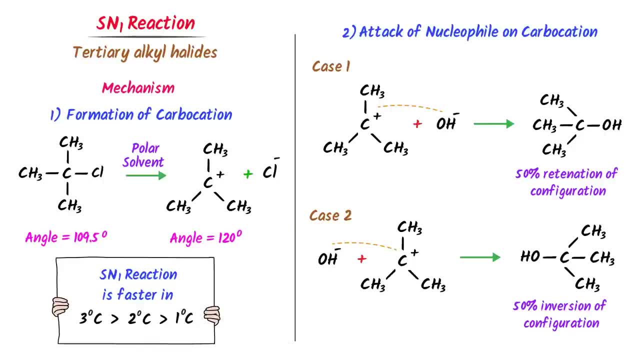 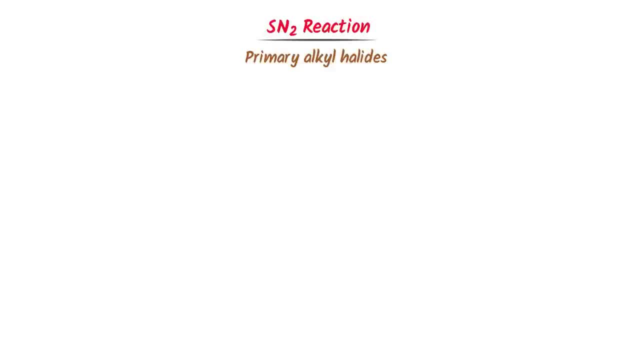 Thus, this is the complete mechanism of SN1 reaction. Now let me teach you SN2 reaction. Remember that primary alkyl halides favor the SN2 reaction. Now I take a primary alkyl halide. I place here a nucleophile. This strong nucleophile will replace this weak nucleophile. 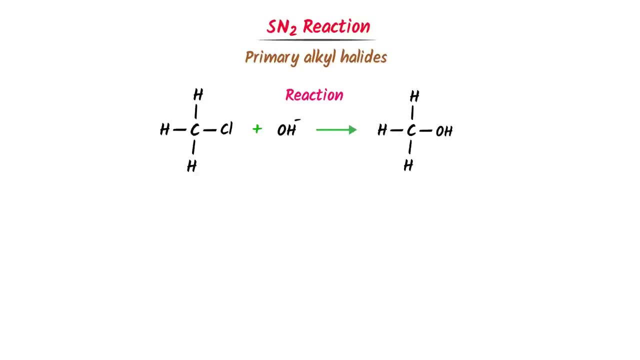 As a result, we get this compound. Now, what about the mechanism of SN2 reaction? Well, it is a one-step reaction, So we get this compound. Now, what about the mechanism of SN2 reaction? We already know that this is a strong nucleophile and this is a weak nucleophile. It is impossible. 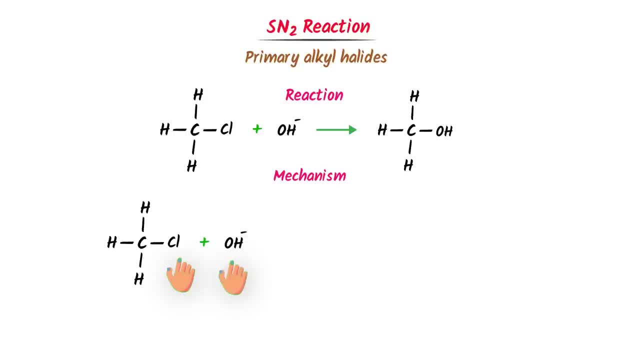 that a nucleophile will attack on a nucleophile. Hence I remove this nucleophile and I place it here. Now this nucleophile will start attacking on this hydrogen. As a result, we will get a transition state. In this state, neither is OH completely bonded to the molecule. 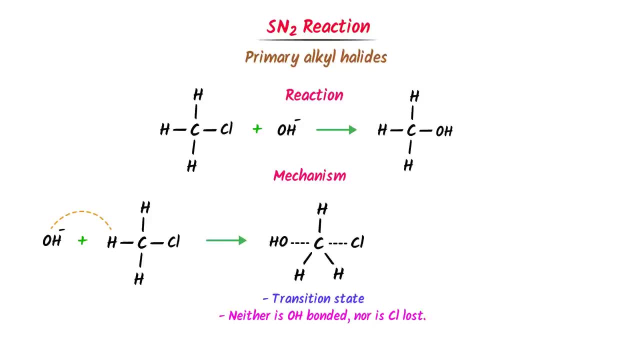 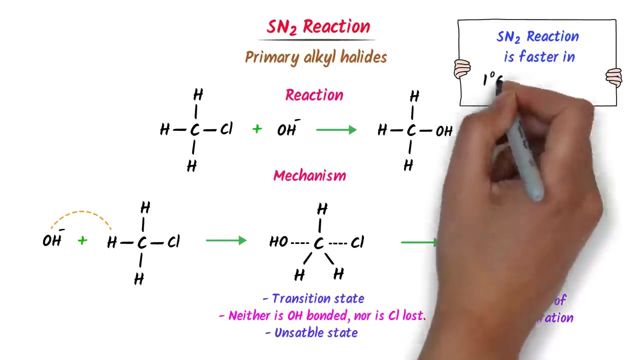 nor is halogen completely removed. Remember that this is unstable state or temporary state. Finally, we get this molecule and the halogen is substituted by OH And SN2 reactions. inversion of configuration occur. Also, remember that SN2 reaction is faster in 1 degree carbon, then 2 degree carbon and then 3 degree carbon. 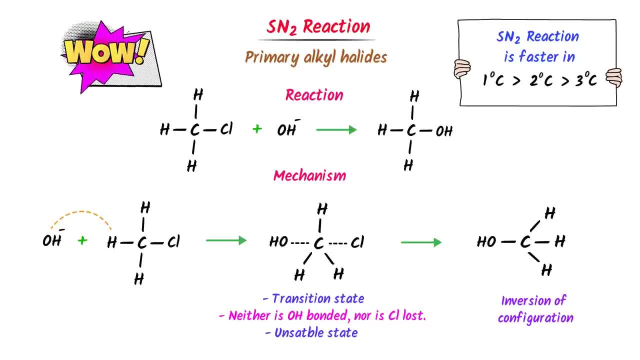 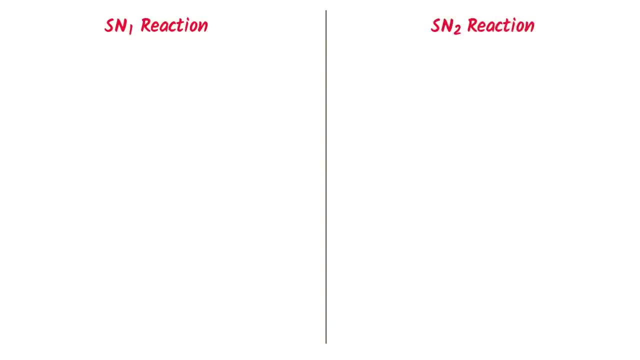 Thus, this is a one-step reaction. Now let me teach you SN2 reaction. As a result, we get this molecule. This is the mechanism of SN2 reaction. Finally, let me teach you the difference between SN1 reaction and SN2 reaction. Well, SN1 is a first-order reaction and SN2 is a second-order. 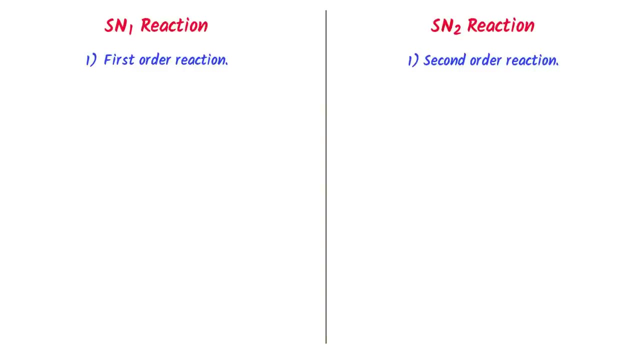 reaction. SN1 is a first-order reaction because rate of reaction only depends on concentration of alkyl halide, While SN2 is a second-order reaction because rate of reaction depends on both the concentration of alkyl halide and concentration of a nucleophile. 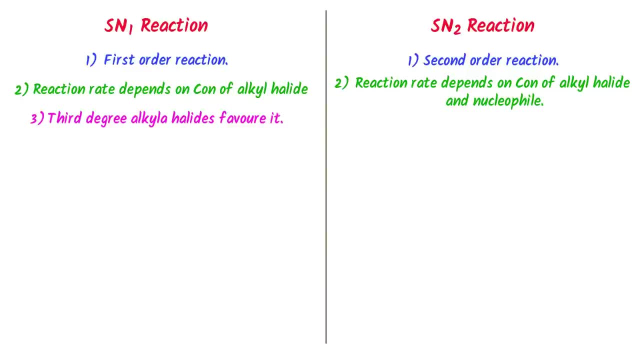 Thirdly, 3rd degree alkyl halides favor SN1 reaction, while 1 degree alkyl halide favor SN2 reactions. Fourthly, it is favored by polar solvents, while SN2 reaction is favored by non-polar solvents. Fifthly, in SN1 reactions, carbocation is found as an intermediate part of SN2 reaction. 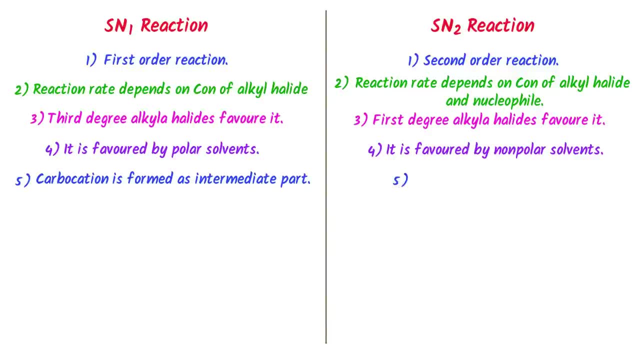 While in SN2 reactions, no carbocation is formed. Sixthly, SN1 is a two-step process, while SN2 is a one-step process. Seventhly, in SN1, rearrangement of products takes place, while in SN2, there is no possibility. 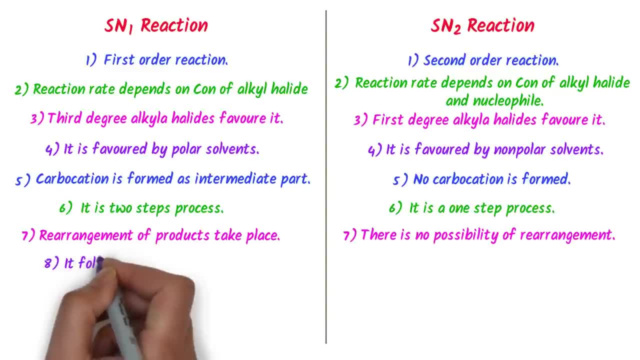 of rearrangement. Eightly, SN1 reactions follow first-order kinetics, while SN2 reactions are followed by first-order kinetics. Ninthly, the nucleophile attacks the carbocation from both the sides, although backside attack dominates, While in SN2 reaction, the attack of nucleophile takes place from the backside.